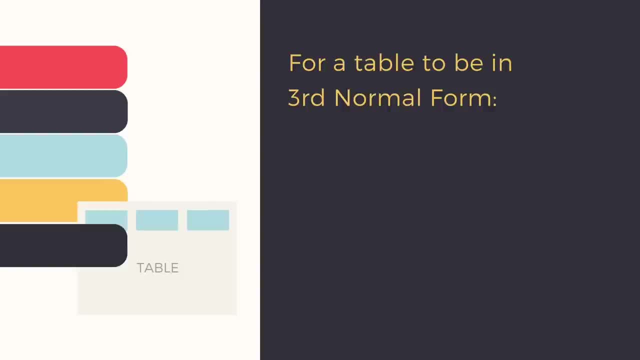 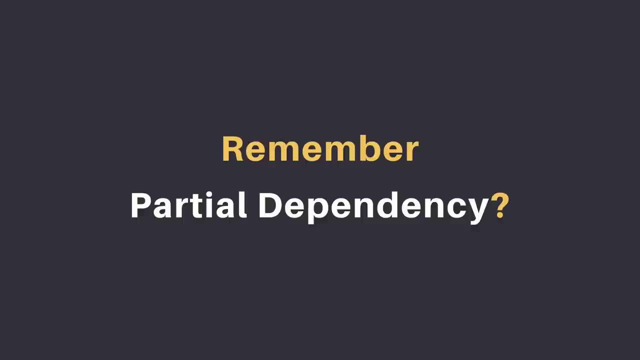 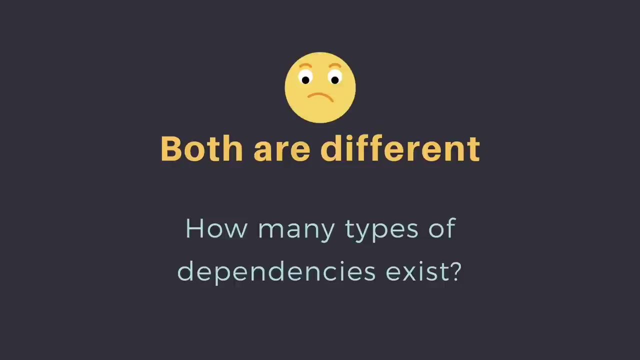 for a table or a relationship to be in third normal form, it must be in the second normal form and it should not have transitive dependency. Remember partial dependency. This time it's transitive dependency. They're different. To understand what partial dependency is once and for all, watch our video. 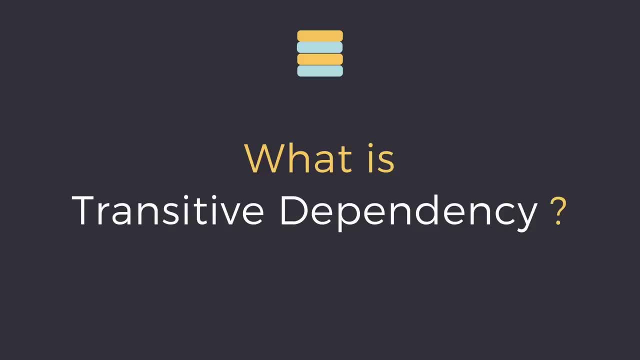 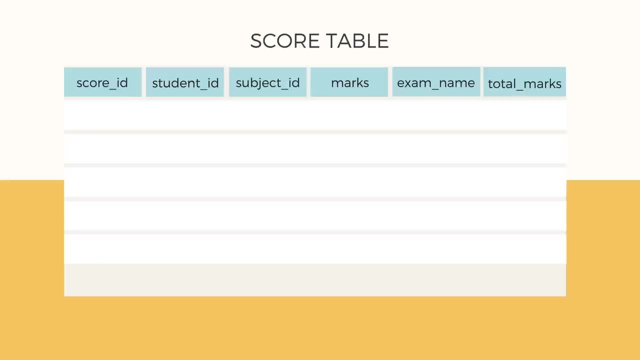 for the second normal form. So what is transitive dependency? With exam name and total marks fields? our score table now looks like this: Primary key for our score table is a composite key, which means it's made up of two attributes or columns: student ID plus subject ID. 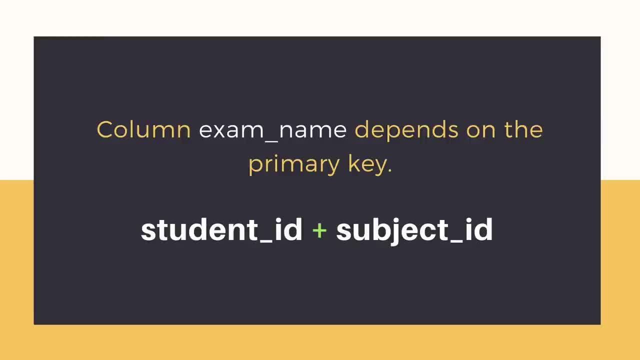 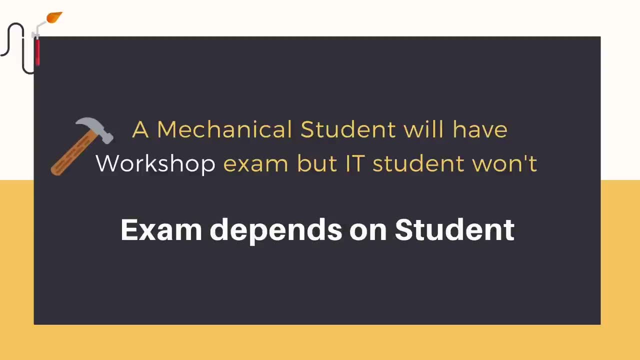 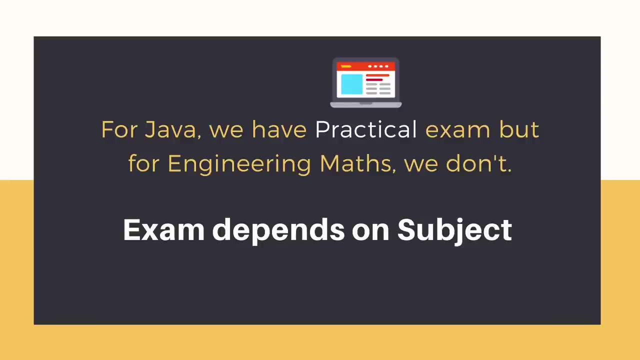 As we can see, our new column exam name depends on student and subject. For example, a mechanical engineering student will have workshop exam but a computer science student won't. And for some subjects you have practical exams and for some you don't. So we can say: 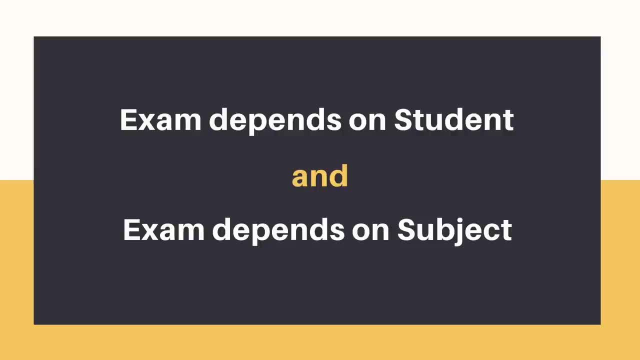 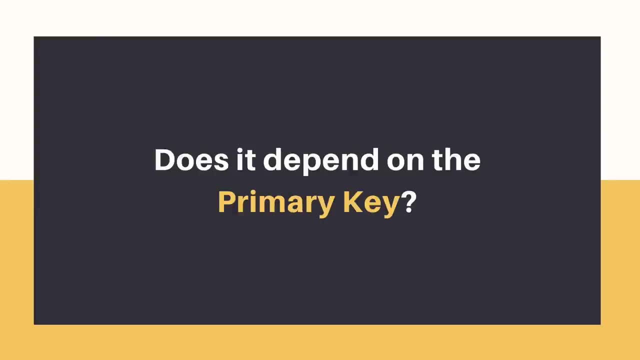 that exam name depends on student and subject, both And our second new column, total marks. does it depend on student or subject, or marks, or the new column exam name? Well, total marks depends on exam name. You must be thinking how, In our colleges, practical exams are generally of 40 marks. 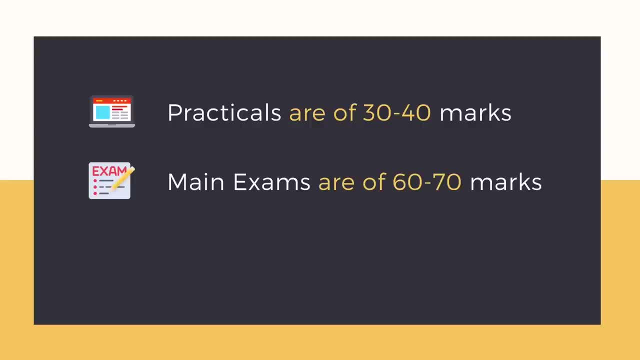 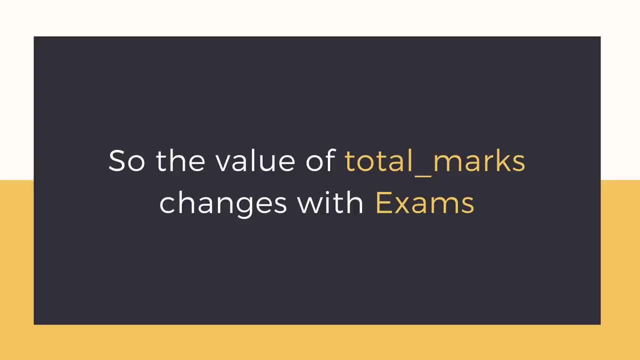 or 30 marks, And theory exams are for 70 or 60 marks. Sessionals are of around 40-50 marks. So all in all, total marks changes based on exam. Hence we can say that total marks depends upon the exam name. Now in our table we already 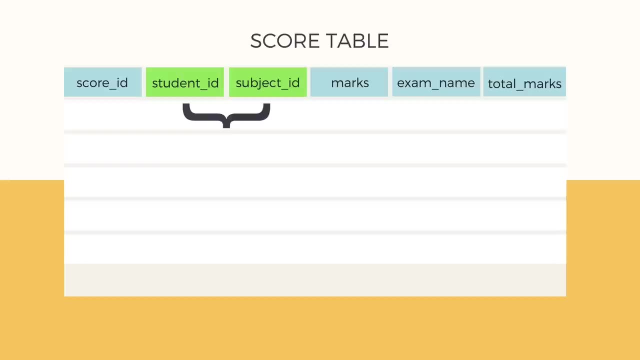 know that the primary key is student ID plus subject ID And all other columns or attributes depends on it, Except total marks, which depends on exam name. But exam name is not a part of a primary key right. This is transitive dependency When there is an attribute in a table. 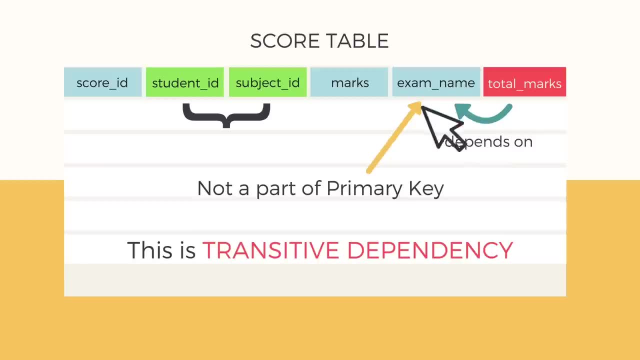 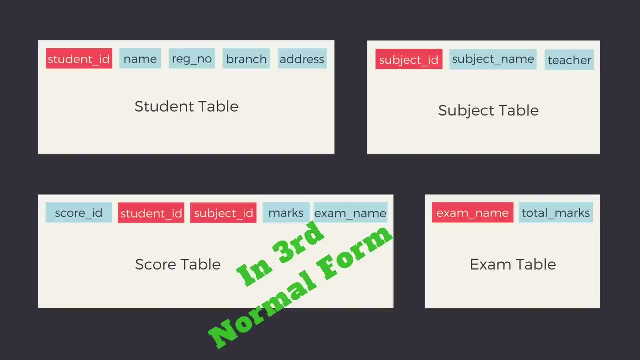 which depends on some non-prime attribute and not on the prime attributes, And the solution to this problem is take exam name and total marks and put them in an exam table and use exam ID wherever required. So now our score table is storing more information and it is in the third normal form.